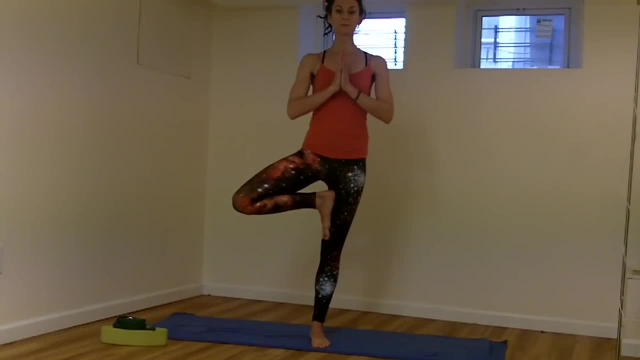 The knee is only an accessory. Keep the hips facing straight forward and use your outer right glute to help you open the knee out to the right. It's more about balance, less about flexibility. Keep pulling up through the core ground, down through your foot and up through the crown of the head. Breathe. 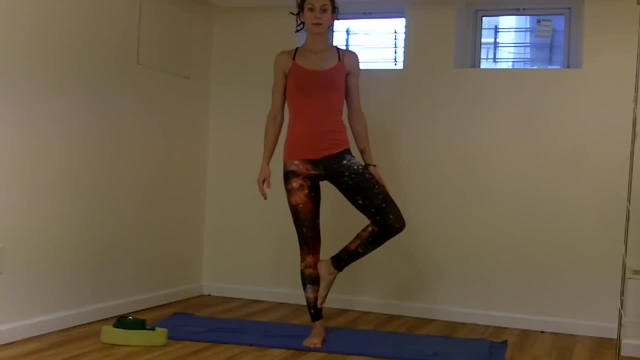 and release Other side Left foot to the right shin or inner thigh, not on the knee. Press the foot into the leg leg into the foot. Lift up through the core, ground down through the standing leg to support the right leg and keep your hips facing straight forward. Use your left glute to 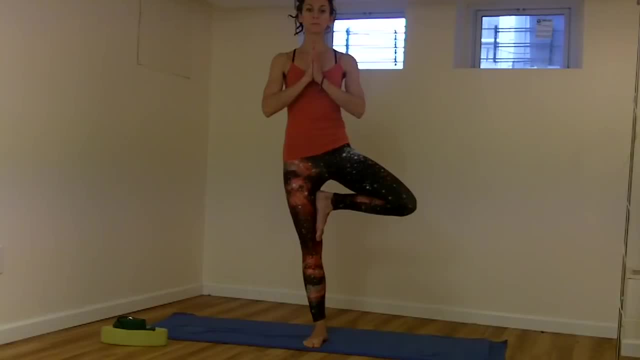 help you open the left knee out to the side. Breathe here, standing tall, feeling the center of your core, really strong Shoulders down your back and you're ready to go. Keep engaging everything towards the midline. Nice deep breaths If you start to waver and wobble. 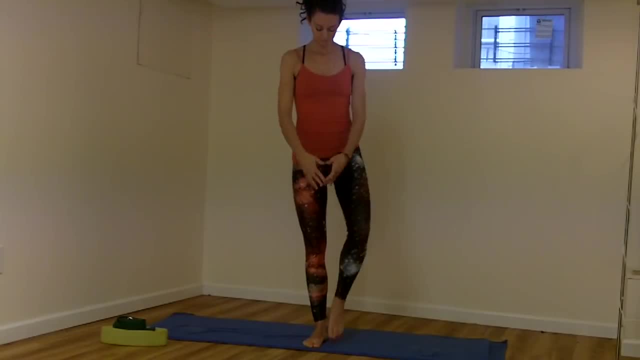 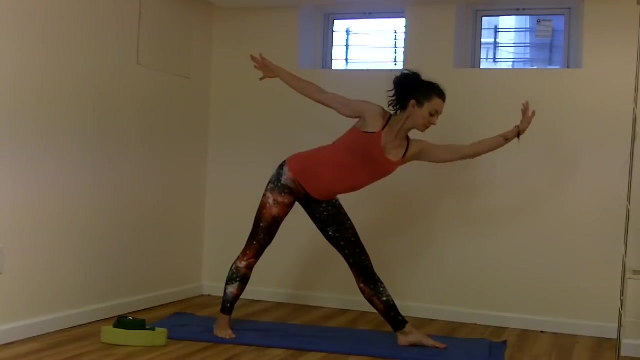 here. that's okay. It's meant to be a balance pose. Release, Step your feet wide and turn the left toes out, right toes in Hands on your hips. Look over your front leg, Shift your left hip back, Reach all the way forward and take your left hand down to your left, shin, Right arm reaches all the. 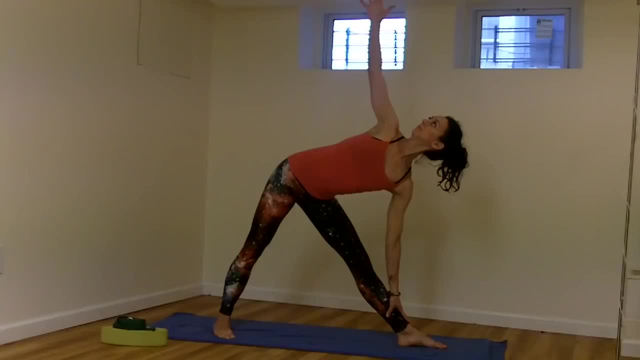 the way up and overhead. The idea here is to drop your left hip back towards the wall behind you so you have a nice long straight line on the left side waist. The right hip presses back, tailbone lengthens and you have a long line from the tailbone to the crown of the head. Keep squeezing. 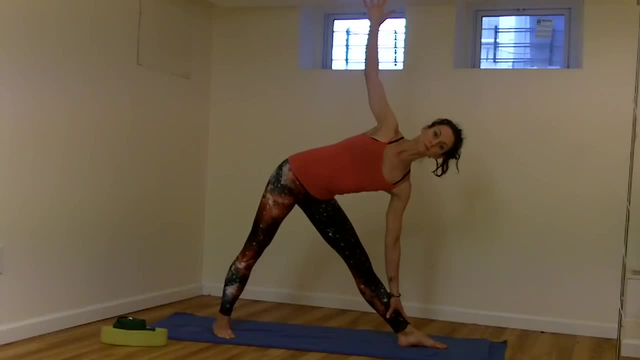 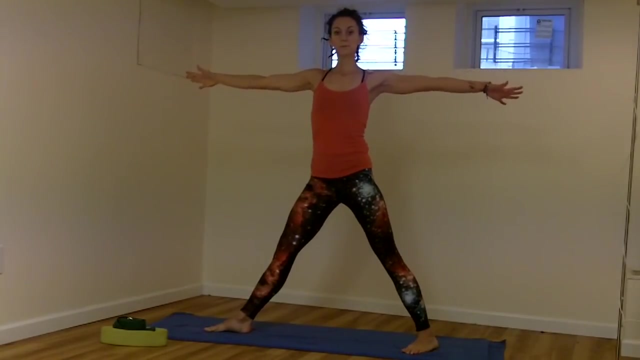 the shoulder blades together and widening through the chest. Imagine you were between two panes of glass. Breathe here, pressing equally through both feet, holding your breath. Come all the way back up, pressing through your back leg. Switch legs Right, toes turn out left. 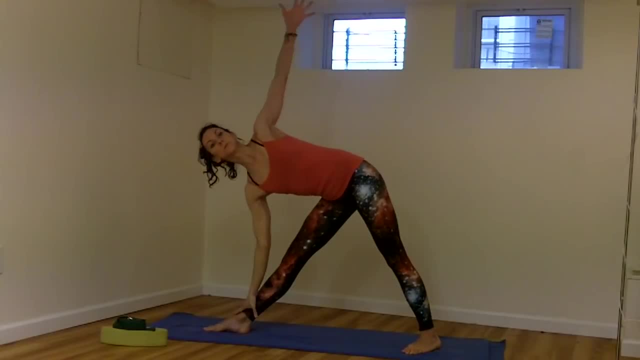 toes turn in Reach towards the right. Right hand drops down to your shin. Same thing here. Push the right hip back towards the wall behind you and lengthen through the tailbone all the way through the crown of the head. Press equally through both feet. 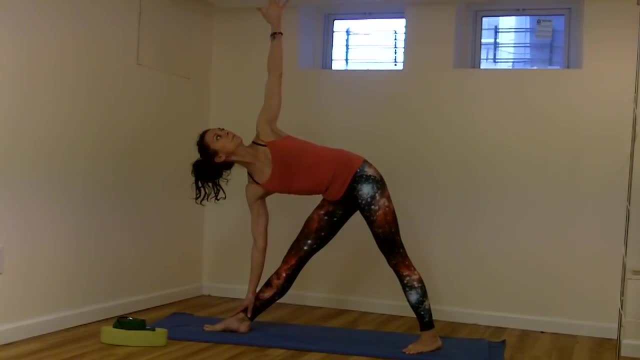 And extend from the tailbone to rotate your chest open, Draw the shoulder blades together, Stay very active in your legs, lifting the kneecaps, deepening through the right hip to lengthen the right side of your waist. Option for the head is either to look forward, 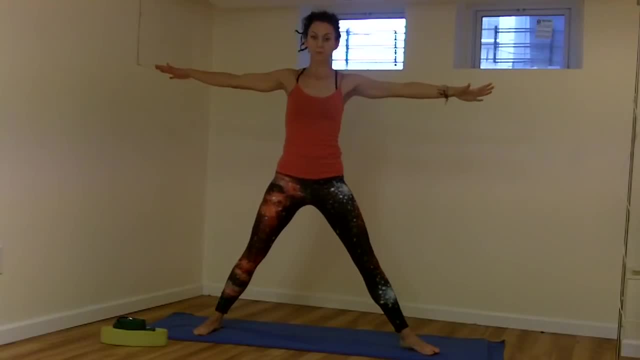 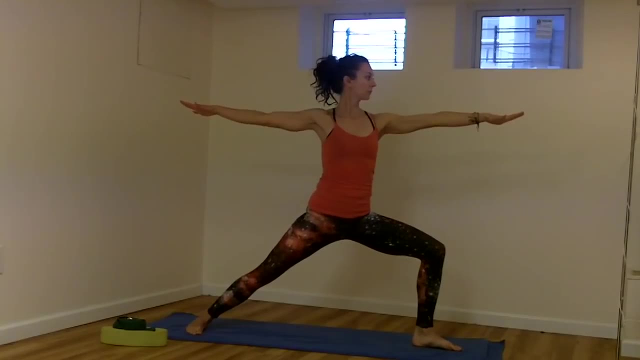 or straight up. Press through your back leg to come up. Widen your stance a little bit further, Shift your weight towards your left leg and come into warrior two. So look down and make sure that your left knee is right over your left ankle and the knee is 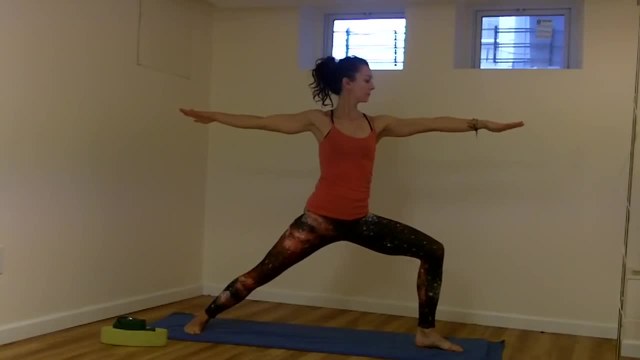 out towards the pinky toe side of the foot, So you should be able to feel this in the left hip. Press out through the back leg. So we're working in oppositions here: Left leg rolls out, right leg presses back. Press down through your hips, but lift up from your rib cage. 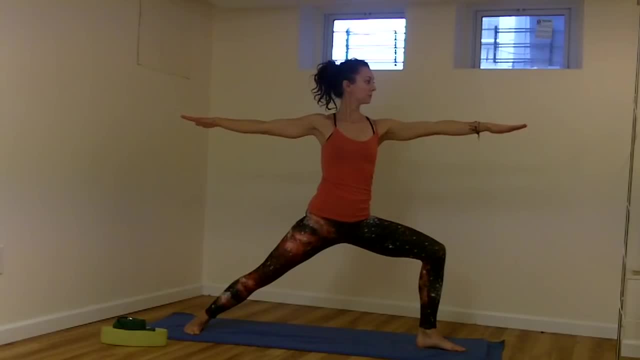 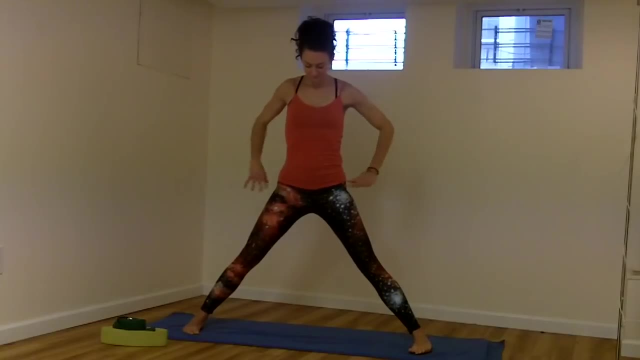 Engage through your shoulders and reach through your fingertips And, if you can go a little bit deeper, Keep breathing Almost there. Straighten your left leg. Turn your feet back to center, Right leg out, left leg in. Bend your right knee right over the big toe of the right leg. 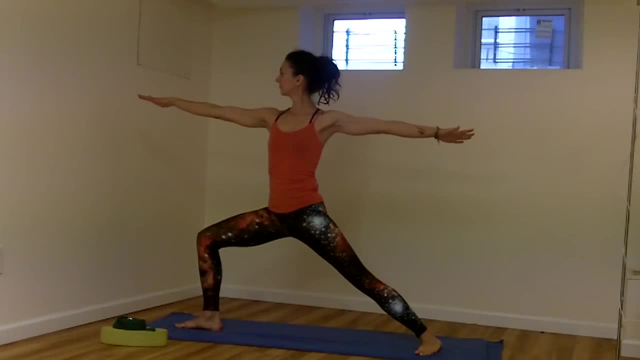 And same thing here. Roll through the outside of your right foot Knee towards the pinky toe side of the foot. Left leg presses back from the top of the thigh. Think of pressing down through the feet from the hips And as you press down through the hips, lift the rib cage off of the hips. 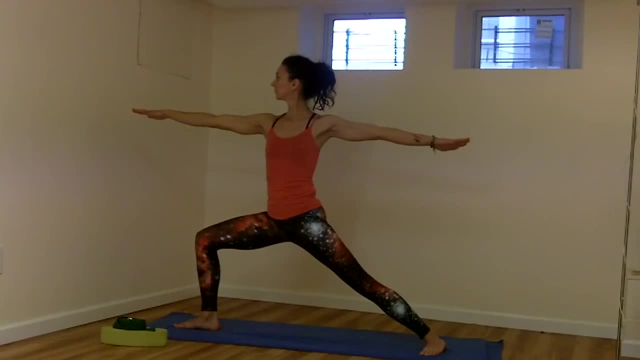 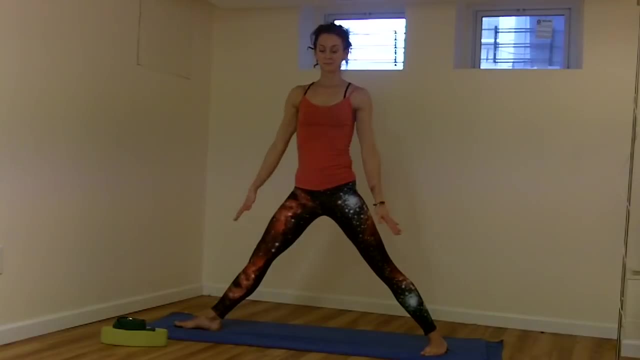 Pull the belly in, Engage the shoulders down the back, Reach through the fingertips and breathe here. If you find that your breath is stopping back off, Straighten your legs. Turn the other direction. Left toes out, right toes in. 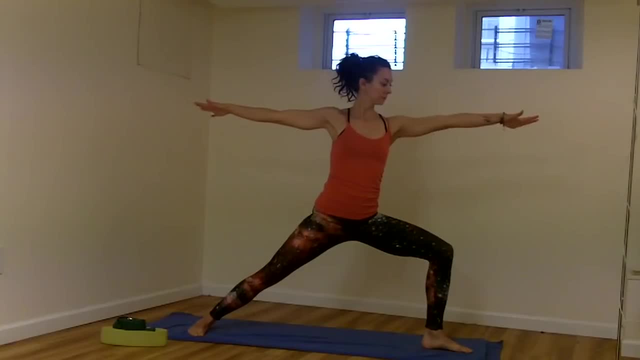 Bend your left knee, Come back into warrior two And then reach your left arm straight forward, nice and long Left elbow down to your knee, Right leg out, left leg in. Bend your left knee, Come back into warrior two And then reach your left arm straight forward, nice and long left elbow down to your knee. 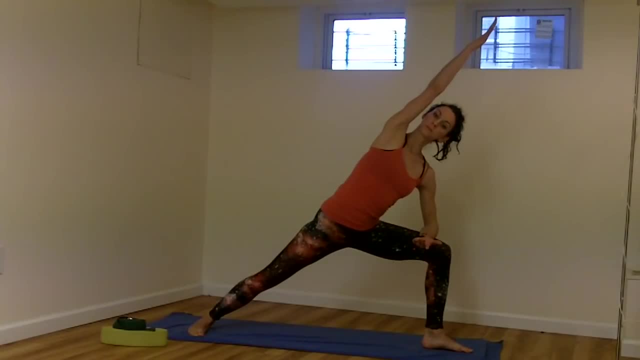 Right arm reaches all the way up over your ears. You want a straight line from the crown of your head to your right heel Option to put your hand behind your left knee on the block, But I like this option too. Firm the legs from the hips, Rotate your chest open, Go deeper, Keep pressing through. 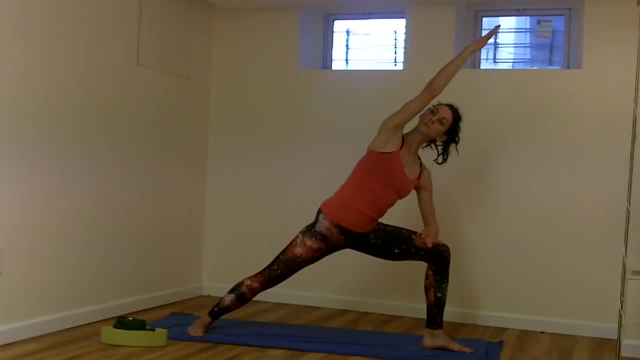 the outer edge of your back foot Core engages to help you open your chest. Nice long line, Deep breaths, See if you can go deeper Again. we're working in opposition, So here. So the front knee bends as the back leg straightens, The left elbow is just lightly on. 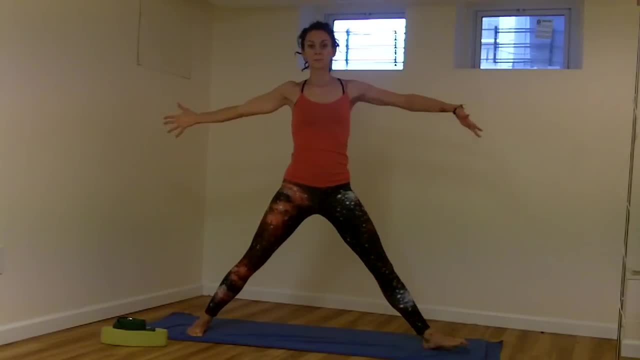 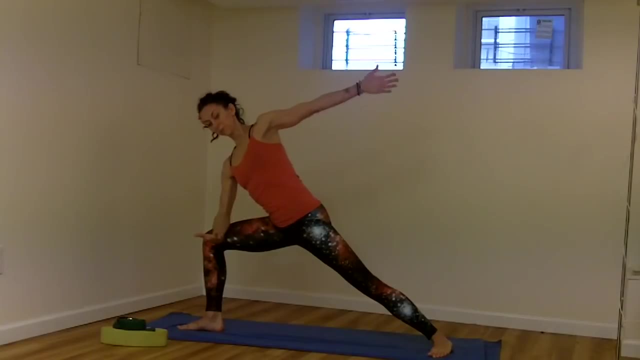 your left knee. The shoulders are opening to the side. Press through your back leg to come up. Right toes out, left toes in Warrior two Reach towards the front, Right elbow to right knee, Left arm reaches up and overhead And then again imagine a straight line from the crown of your 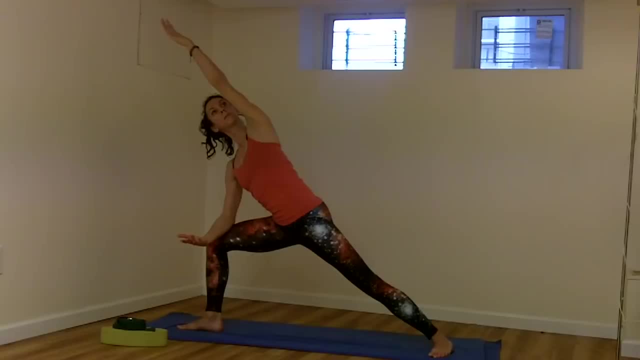 head to the left outer heel. Press the right knee towards the pinky toe side of the foot and the left thigh back towards the wall behind you. Engage your core to help you open your chest and remain light on that right elbow on your knee. Breathe here Nice, deep breaths. 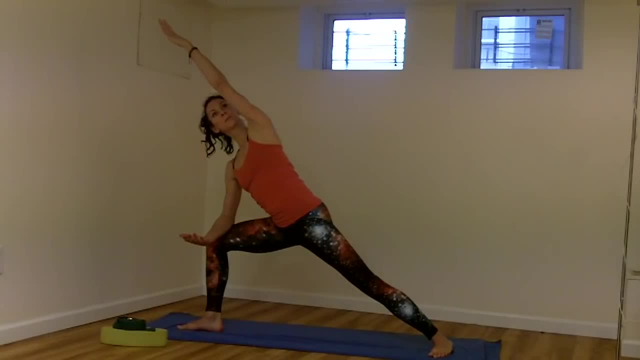 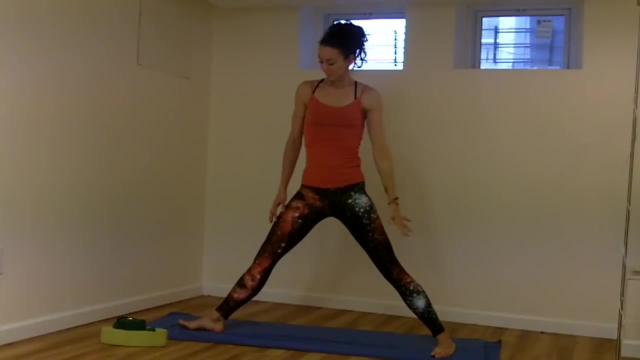 If it starts to get challenging, start to deepen your breath a little bit more, Press through the back leg to come all the way back up And then grab your block and swivel your feet all the way to face forward and take the block on the inside of your left foot. 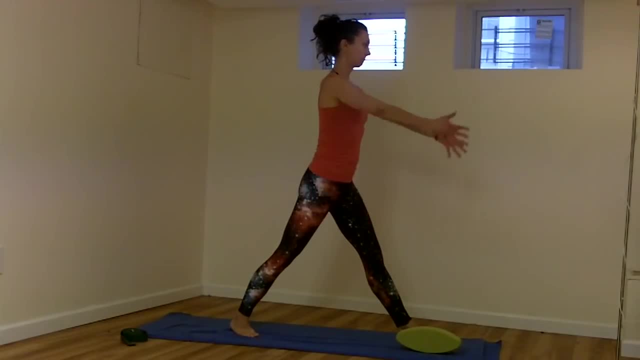 And pivot your feet forward so your right heel is on the ground. Lift both arms up overhead. Take your left hand into your right hip to help pull it back and then reach all the way forward with your right hand down to the block. Come up to the block, Lift your chest flat. Press through the 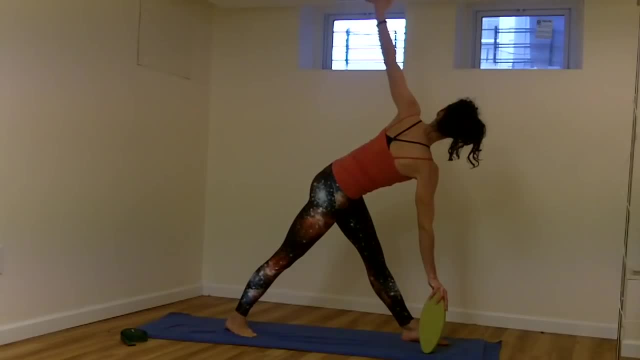 back leg to come all the way back up And then grab your block and swivel your feet all the way back up And then open your left arm towards the ceiling, coming into a twist. Press equally through both legs, the right heel and the left heel, sending the left hip back towards the wall. 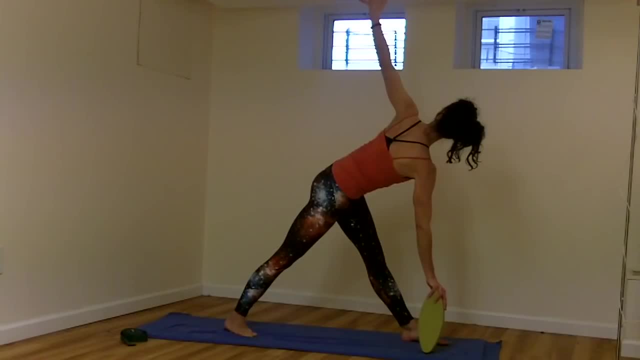 behind you, Roll your shoulders open, Find the twist from the core And see how long you can get from your tailbone to the crown of the head. Press down through the feet, out through the core, rotating through the chest. Deep breaths here, The deeper the breath. 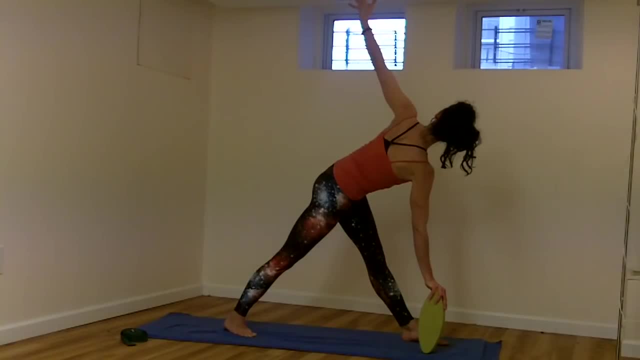 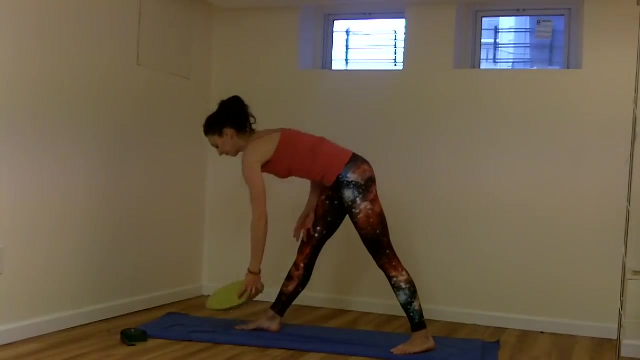 the more you can go into the pose. Take your left hand back down, Come all the way up. Swivel your feet to the other side. Right foot turns out. Left toes turn in. Block on the inside of the right foot. Lift both arms up overhead Right. 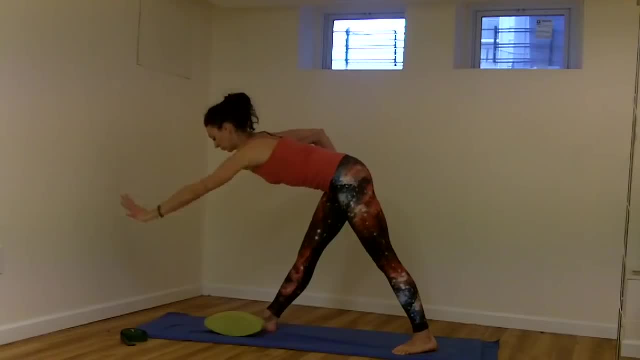 hand into your right hip. crease. Reach all the way forward to lengthen Hand down to the block. Square your hips so the right hip is on the ground And then come all the way up. Swivel your feet to the side- Right hip is pulling back. Press both legs down And then open your chest towards the front. 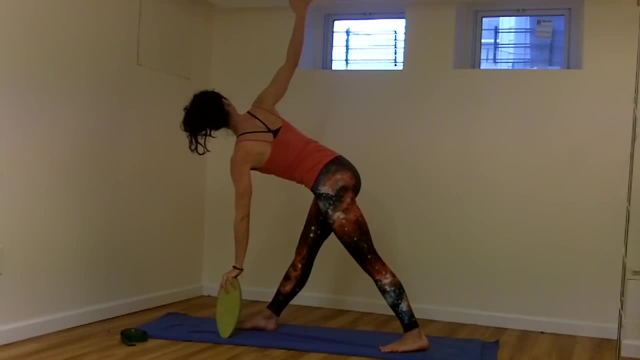 leg. Keep the legs really straight. Press down through both legs, Pull that right hip back towards the wall behind you And use your core to help you twist your chest open Shoulder blades, pull down the back And you have a long line from your tailbone to the crown of your head. 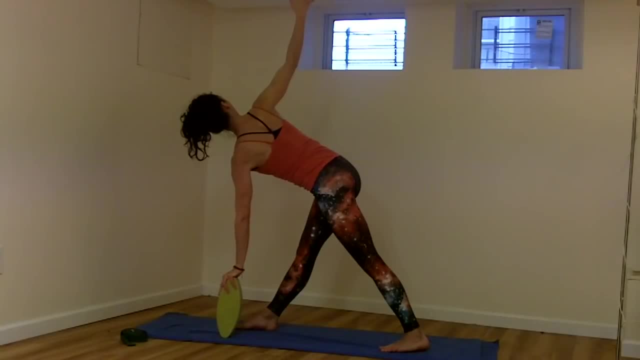 Stay steady here with your breath. Legs are strong, Quads are active, Hips are even. Find your strength in your legs. Breathe deeply into your core And then see if you can twist a little bit more through your upper back. Squeeze the shoulder blades together. Drop the right hand. 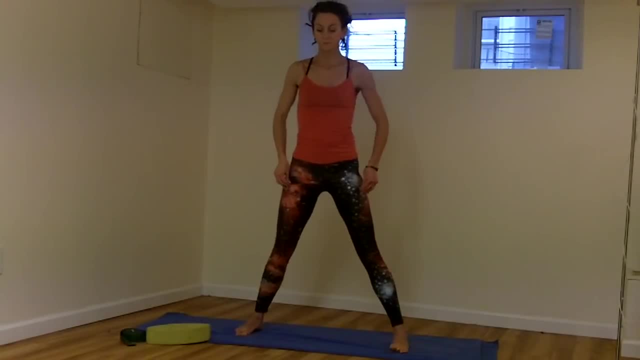 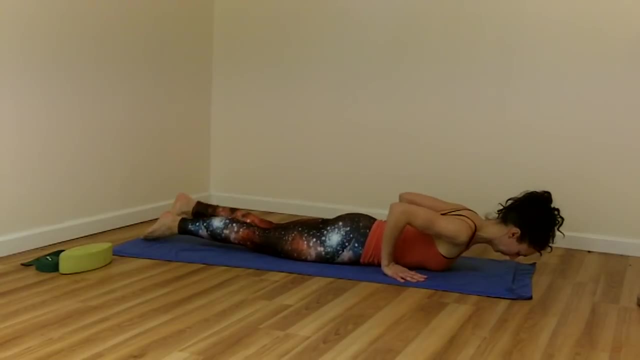 Press through your back leg to come all the way back up And we'll come down to the floor. From hands and knees come all the way down to your chest. Hands underneath your shoulder, by your ribcage. Press your hands down, Lift your chest, but don't arch your neck all the way back. Reach. 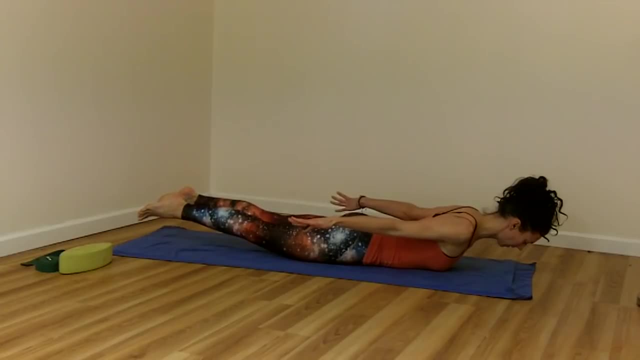 the arms all the way back, Legs off the floor. Shoulder blades should be pulling down your back like you are trying to reach back to touch your toes. Neck stays nice and long Legs are lifting from the backs of the thighs and reaching through the toes. If you feel this in your lower back, 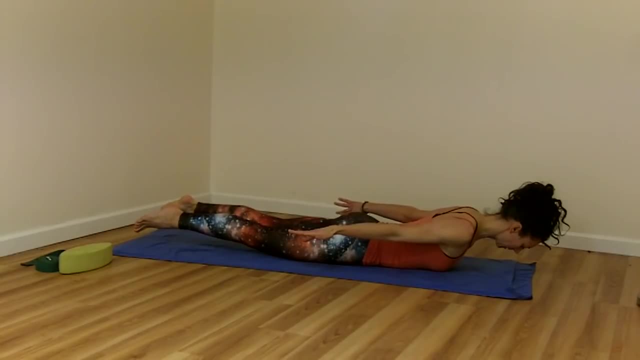 you might come down a little bit. Engage your core and tuck your pelvis so that the pubic bone is sitting Into the floor. It'll help lengthen your lower back. What's more important here is the length from the crown of your head to your toes, not so much the height. Keep breathing nice. 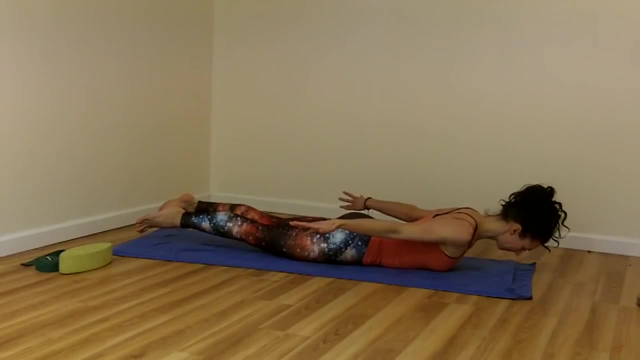 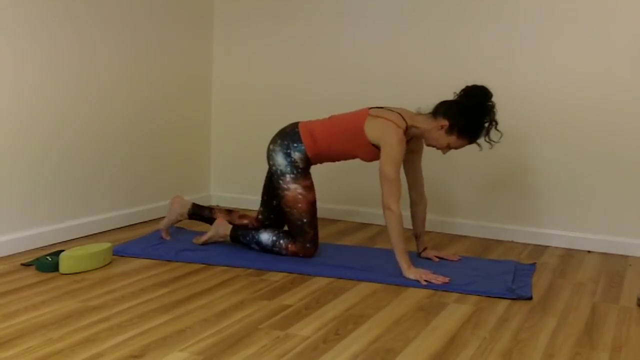 deep breaths, Squeeze the shoulder blades together right from where your shoulder blades meet, So not in the neck, but a little lower- And then lower down. Turn your head to one side, Take a couple breaths, Press back to all fours and then come to lay on your back. 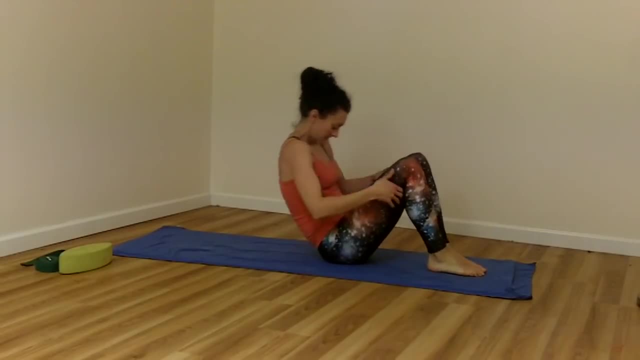 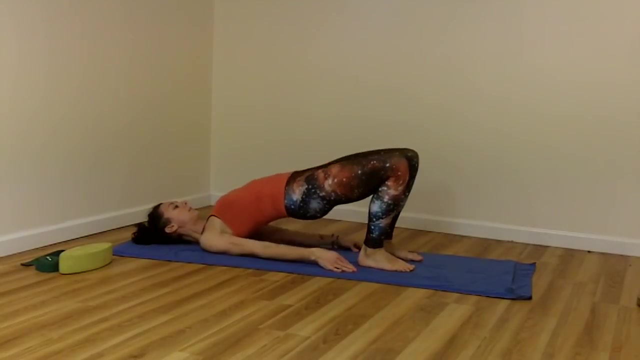 Roll down one vertebrae at a time And then move your heels as close as you can towards your hips, Press your hips towards the ceiling, Roll your shoulders underneath you and then interlace your hands underneath your back. So what's important here is not to move your head. Keep pressing the 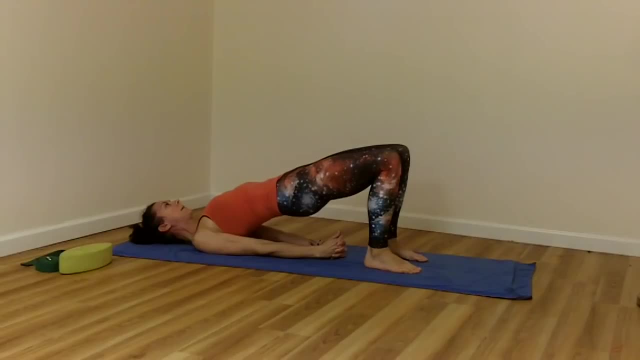 back of your head into the floor. Roll your upper shoulders down and back into the floor And use your upper arms to press into the floor. Drive your heels into the floor And internally rotate your knees in towards each other. So again, if you feel this in your lower 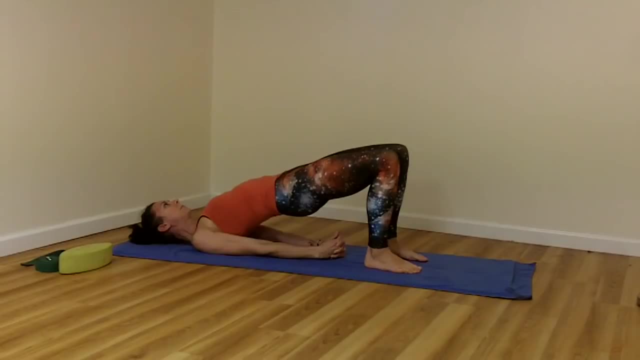 back. you can press the tailbone towards the ceiling, almost like tucking your tailbone a little bit. These full, deep breaths here- And there's a lot of activity going on here, Pressing through the legs, Pressing through the arms, Breathing into the chest- Stay with it, Breathe. 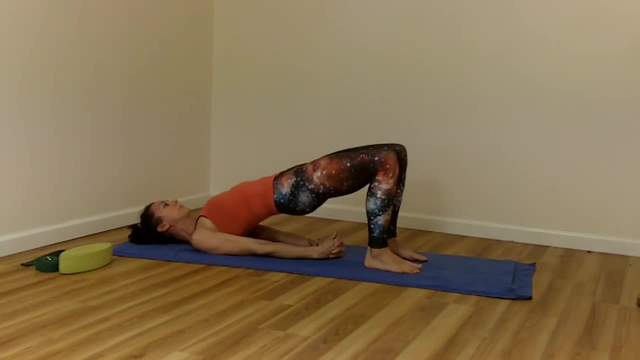 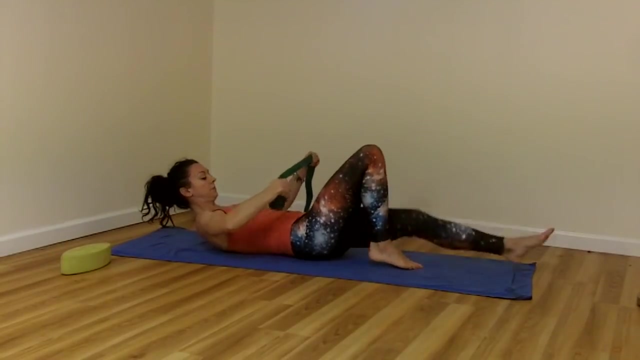 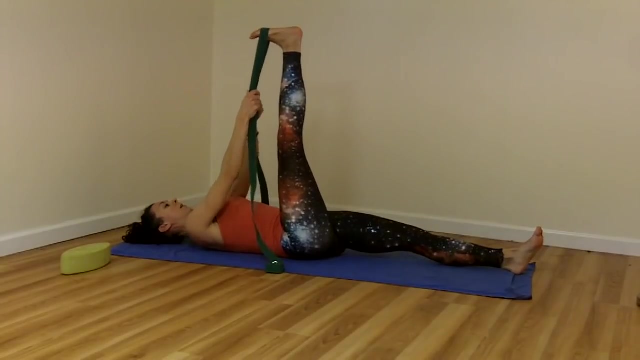 through it. Release your hands, Lower your hips down to the floor And then grab onto your strap or towel or belt And we'll take the strap around your right toes, Straighten the right leg all the way towards the ceiling. If you need to bend your knee a little bit, that's okay too, as long as you feel. 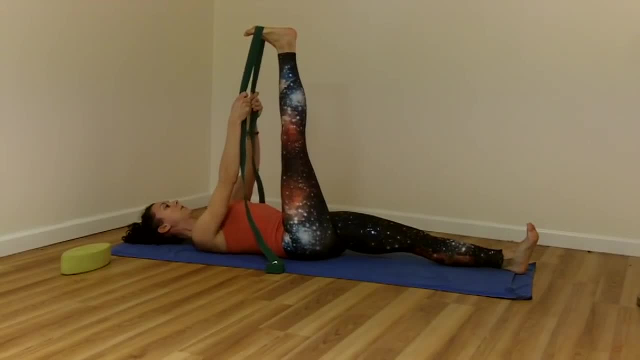 it in the belly of the hamstring. Hold on to each end of the belt with one hand And then press the right hip towards the wall in front of you. You want to lengthen the right side waist. We're going to stay here for 30 seconds. Keep activating through the left leg internally. 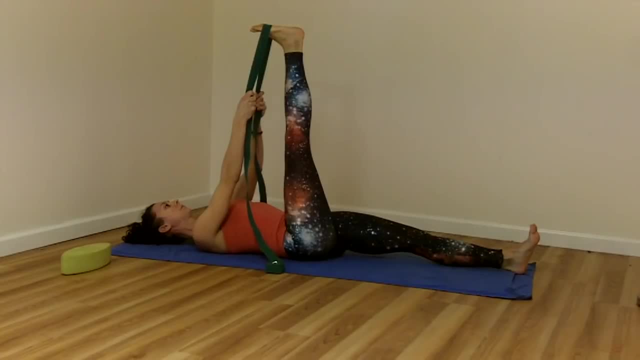 rotating it, almost like you're rotating the toes towards the ceiling. Lengthen equally through both legs And then ground your shoulder blades down your back as well. It's a very active stretch. Breathe, Find your breath And again, if you're feeling it too much in behind the knee, you can bend the knee. Take both ends of. 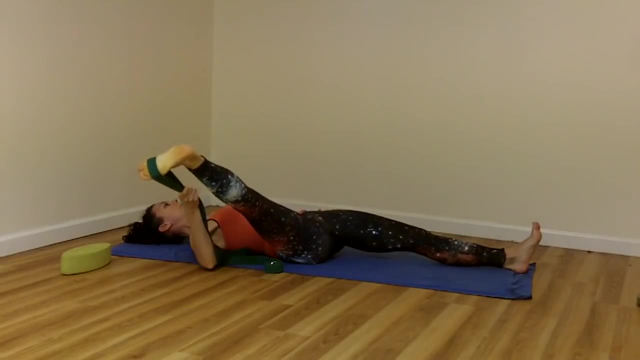 the belt in your right hand and slowly take the right leg out to the side, making sure that you keep the left thigh pressing down towards the mat And pay attention to your shoulder blades here. Make sure your shoulder blades are released down onto the floor. 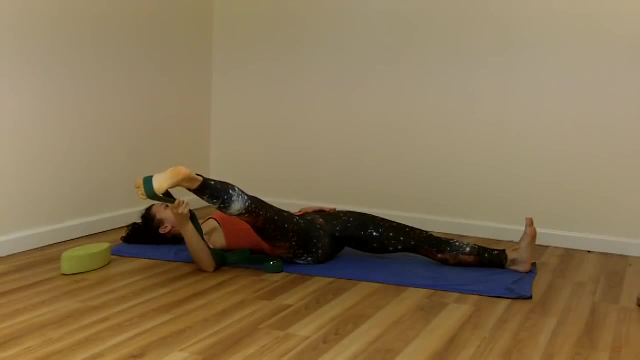 It's okay to bend the knee. that's in the band. Make sure you can also feel this in the inner thigh and in the hamstring and not in the attachment up near the tailbone. Keep pressing that left thigh down. Left foot is very active- And then keep pressing the right hip towards the wall in front of you. so 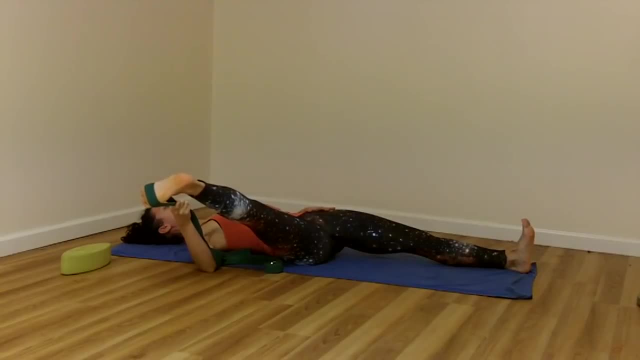 you're deepening that right side waist And then coming all the way back up to the side. Now lie down Back up to the center, Switch hands with the belt so the left hand takes the belly. Take the leg over just a couple of inches. 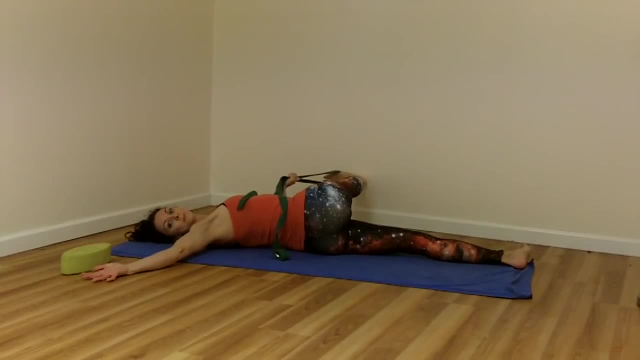 Like five or six inches from here. Drop your right hip towards the floor and then take the leg all the way over to the side. drop that right hip forward, Roll it forward and then extend the right arm out to the side. Look over your right shoulder. The right leg is straight or slightly bent. 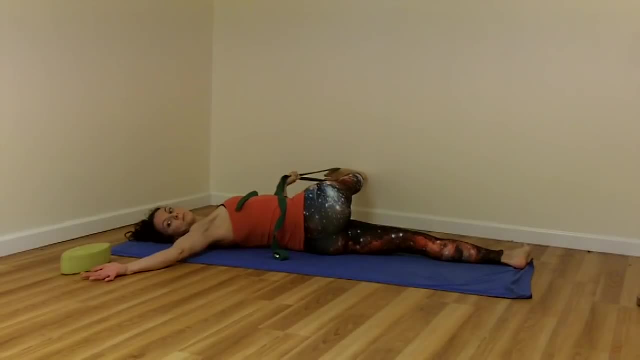 Press your big toe mound in between the feet, bringing your thumb in and kicking it up, And situationally attack with a punch, even if your hand is cleared off by your hands on the ground. Press your big toe mound into the belt so you're extending through the 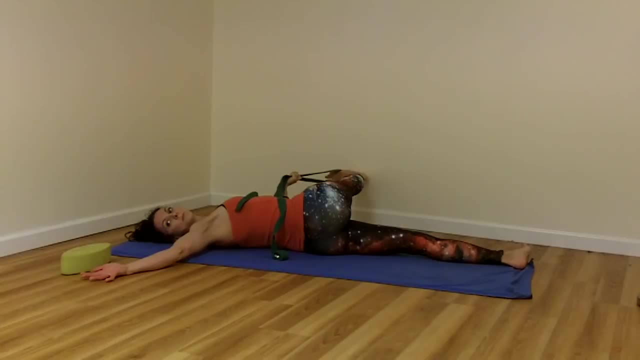 inside of your leg. It will help fire up the stretch in the outer hip. You can breathe right into the core here to help you accentuate the twist. So you're still remaining active, The foot is off the floor, Kind of an active stretch. 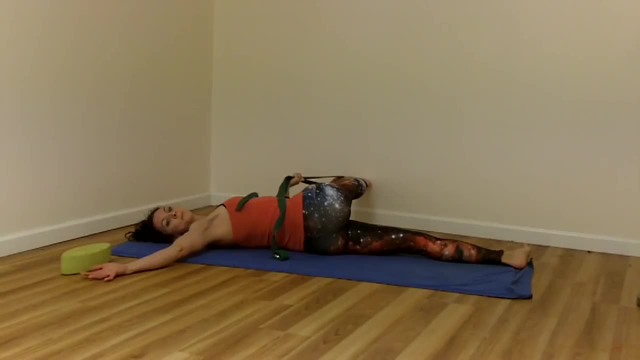 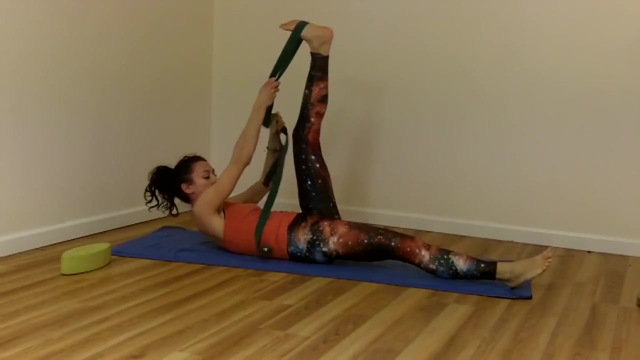 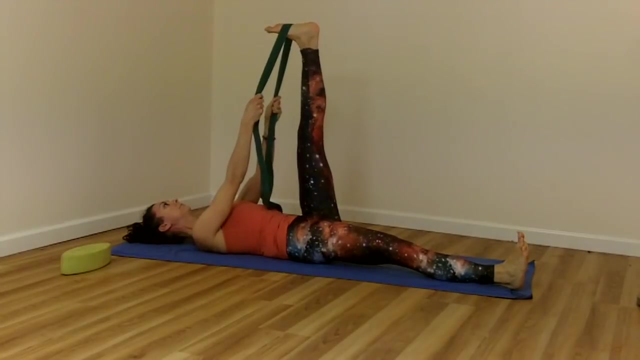 Nice, full, deep breaths And then bringing it all the way back to the center And we'll switch legs. Left foot in the belt, Right leg extends, And then take one end of the belt in each hand, Anchor your shoulders down your back and then straighten both legs as much as you can. 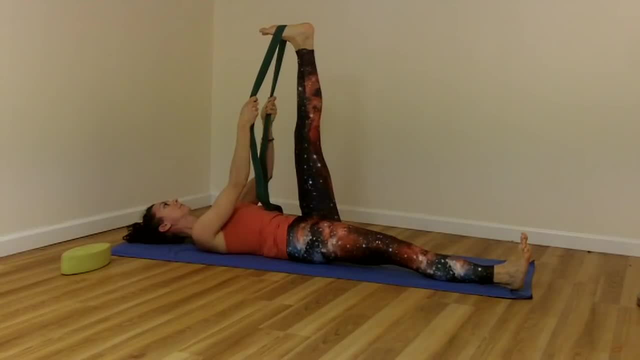 If you can't straighten it, that's okay. I would rather see it a little more forward than too far forward. and bent Good, Press through the right leg, Drop your left hip towards the wall in front of you. So what I mean by that is, if you. 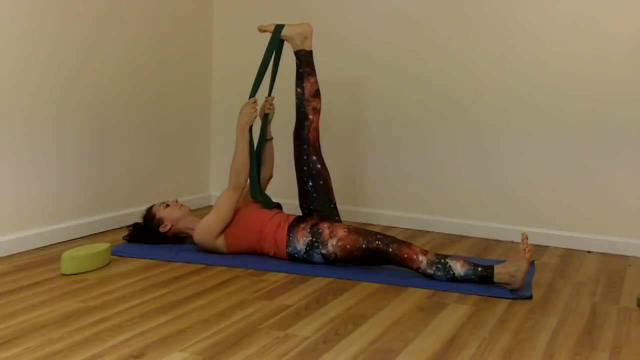 feel like you can't straighten your leg all the way, it's okay to keep it bent. Keep breathing Nice, solid, deep breaths. I'm going to take both ends of the belt in your left hand. Keep the right thigh grounded on the floor as the left leg goes out to the side. 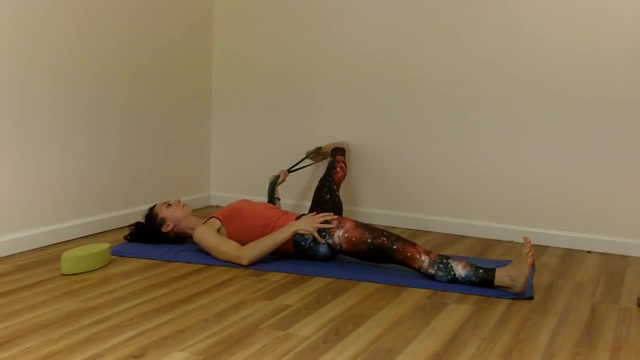 Not all the way to the floor, Only as far as you can go without lifting the right hip off the floor. You're staying very active through. the right leg Core is pulling back And the toes are slightly rotated towards the floor- The toes of the left leg. 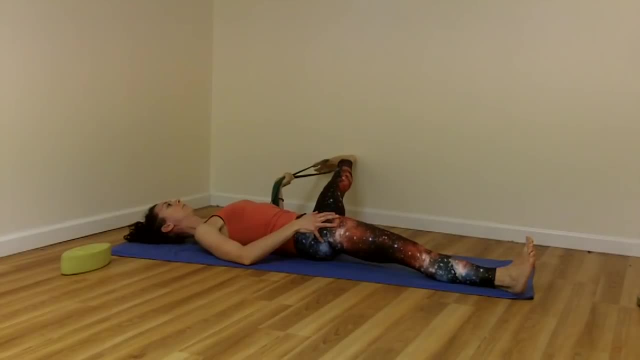 The leg in the belt. Inhale and exhale. Feel the sensations of your legs. Press through the right leg. Keep the toes pointing towards the ceiling. Core is active. Lift the leg all the way back up to the center. Switch hands with the belt. Take the belt all the way over to the right about six inches. 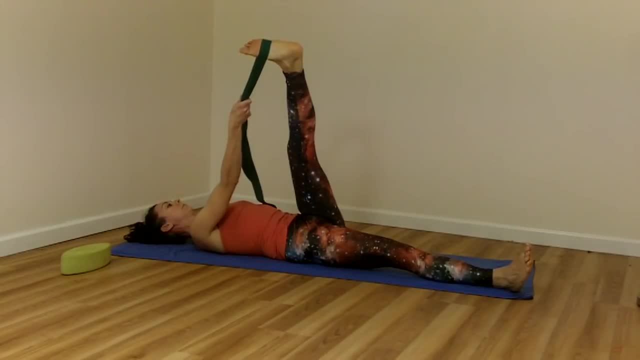 You'll feel the muscles in your legs. You'll feel the muscles in your legs. You'll feel a major stretch here And then go all the way over towards the right. Let your leg come all the way down. Keep it off the floor. 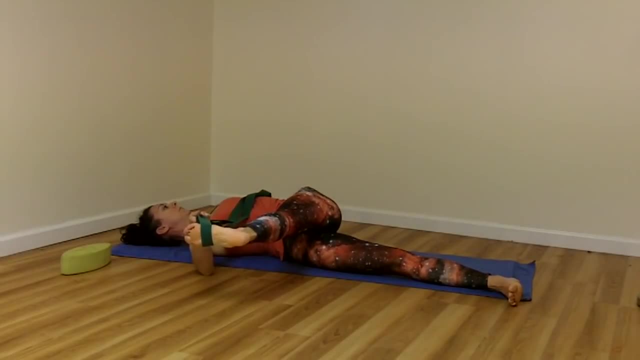 Drop the right or the left hip towards the wall in front of you And then press the big toe mound into the belt. So you're thinking of dropping the left hip towards the wall in front of you and then pressing through the big toe mound. 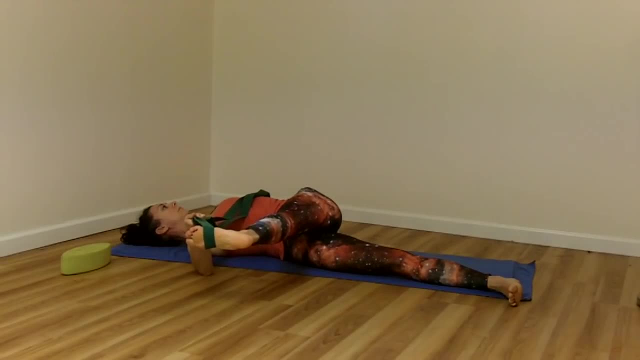 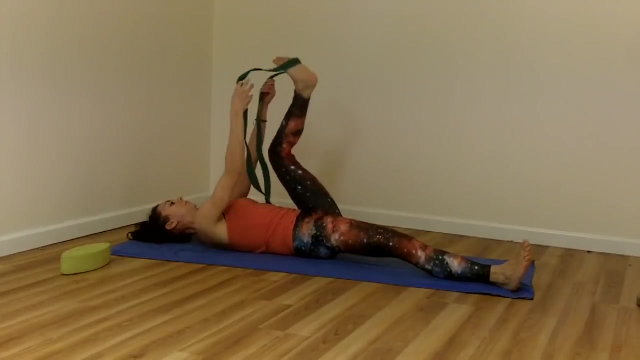 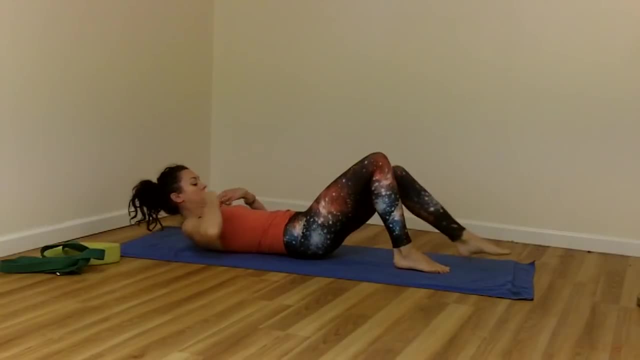 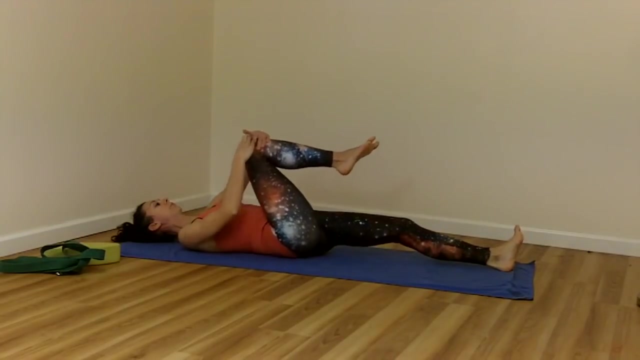 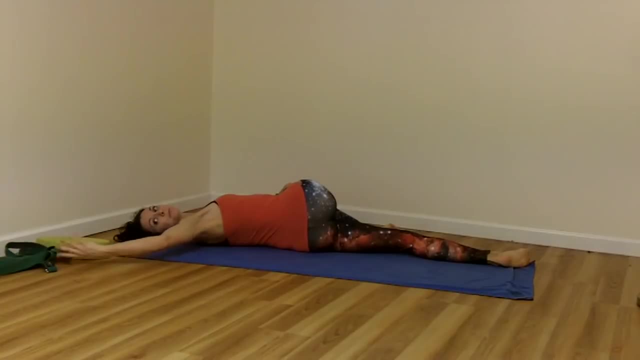 So you can roll all the way to your left and then open the arm out to the right So that left knee is fully on the floor. Press the left hip towards the wall in front of you And let the breath deepen, the twist from your core. 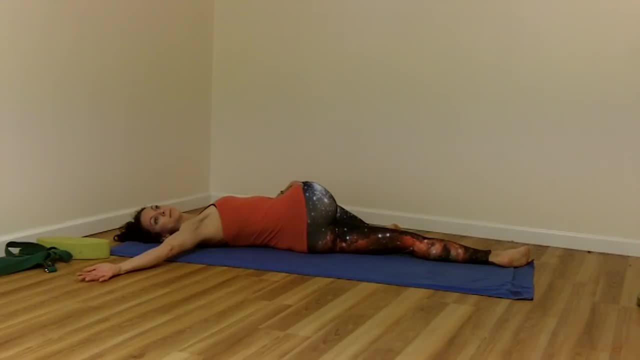 And the longer you stay in this position, the more you're going to be able to relax. And the longer you stay in this position, the more intense the stretch will become. You might feel this in the right shoulder, But the more you do it, the more that right shoulder will open. 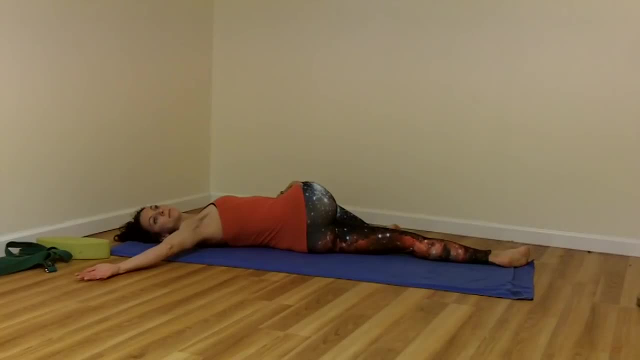 And there's still a little bit of activity here. Press the right hip away from your shoulder Shoulder down into the floor And breathe Long, solid breaths. Breathe in And breathe out. Breathe in And breathe out. 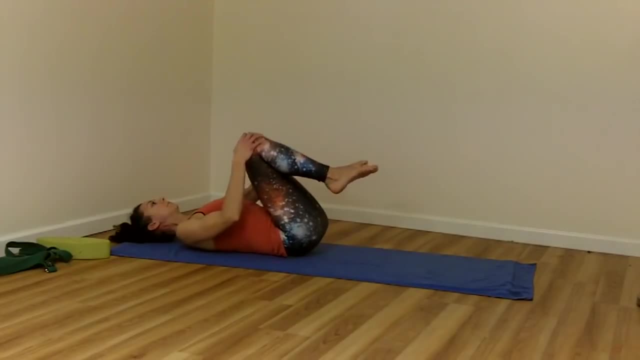 Bring your right knee back into your chest, Bring your left knee up to meet it- Right leg extends. Flex the foot on the floor And then take the left knee across your chest all the way to the right And shift that bottom hip under. 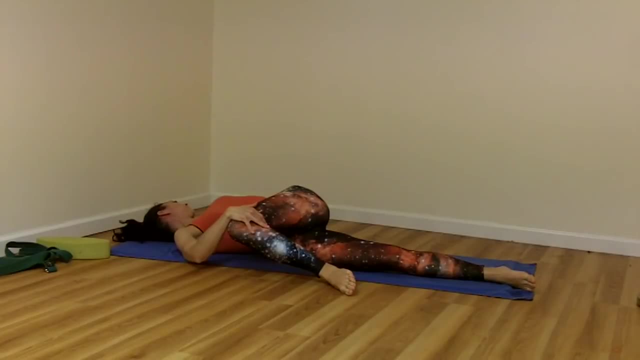 And then open your chest to the left And again drop that left hip towards the wall in front of you. Deepen the twist from your core And then let your left shoulder open naturally from your chest. Breathe, Breathe into any of the sensations that you feel. 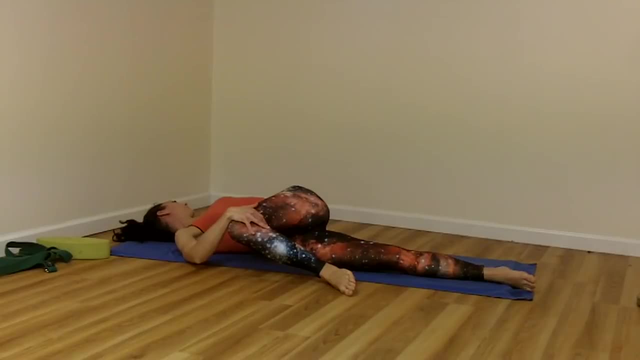 Any tightness or holding. See if you can send your breath there and soften. So while we're working here, we're also working to release. Breathe in, Breathe out. Bring your left knee back into your chest. Hug both knees into your chest. 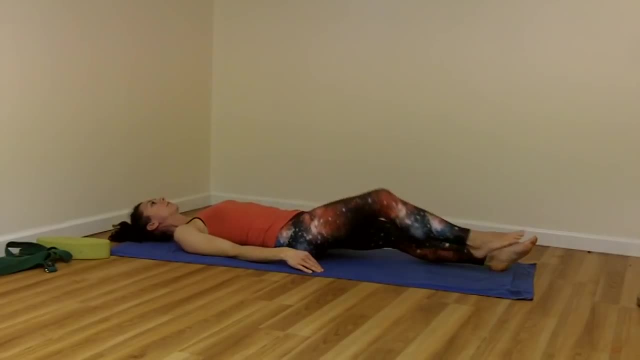 Press your hips down, Knees in And then set yourself up for Corpse Pose. Let your arms relax out to the sides, Let your legs fall apart, Let your head be heavy on the floor And fully relax. Let go of all of your muscles. 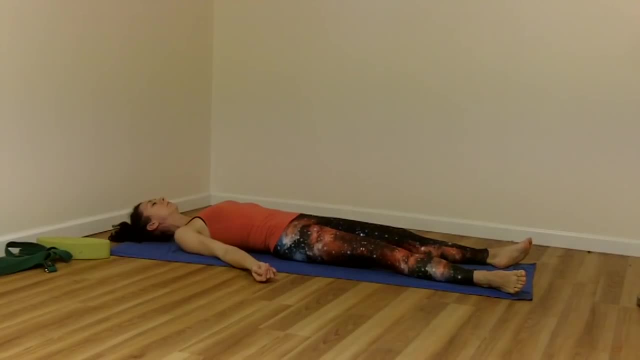 Let go of all of your muscles. Follow your breath. Just let your breath be normal. See if you can completely and totally let go. If your mind starts to wander, just go back to your breath, Watching your breath go in and out.